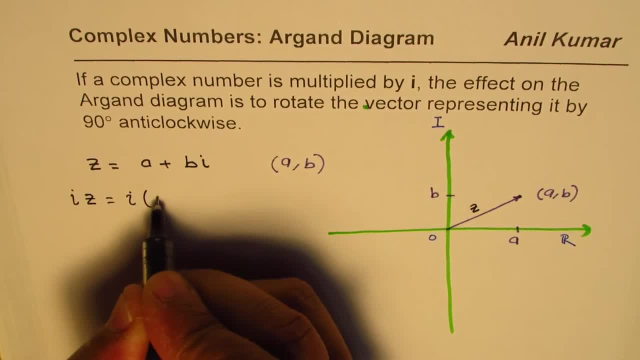 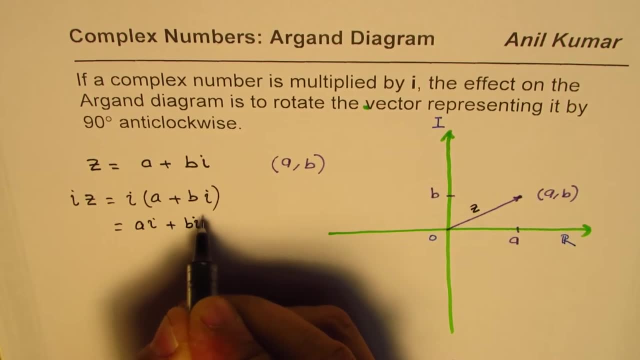 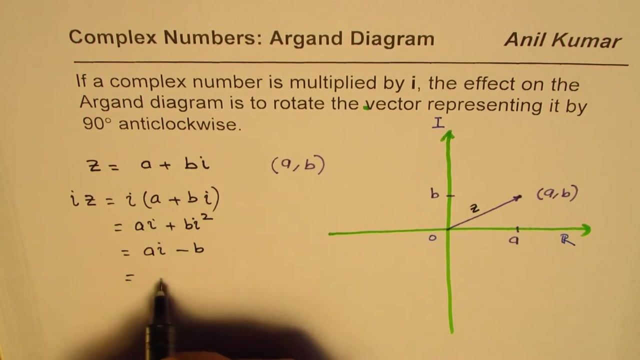 let's have a look. so i times z is i. times a plus b i expanding, we get a i plus b i square. i square is negative one, so i could write this as a i minus b and rearranging i write minus b plus a i. right, so it becomes minus b plus a i, which could be represented now. 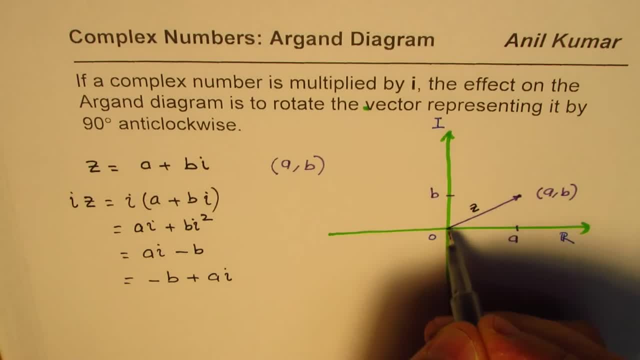 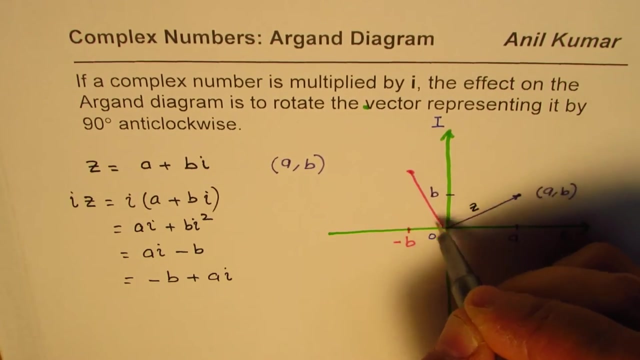 on the same organ diagram as minus b, so that much of unit i'm taking along this direction. so this is minus b a along the vertical axis. so this much unit i'm taking along kind of here. so that becomes the point and this arrow joining with the origin represents the complex number. 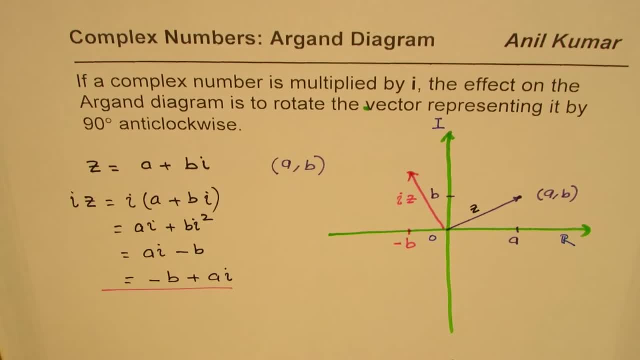 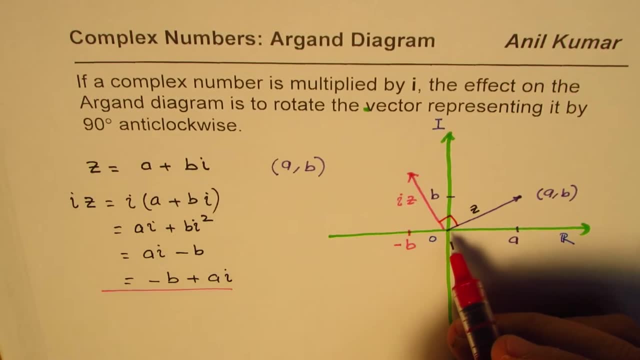 i times z, it looks as if it has rotated counterclockwise by 90 degrees. how can we be sure about it? well, let's find the the angle right. so in this particular case, in the first place, let's say: this is point a, And here we go to point B from the origin. 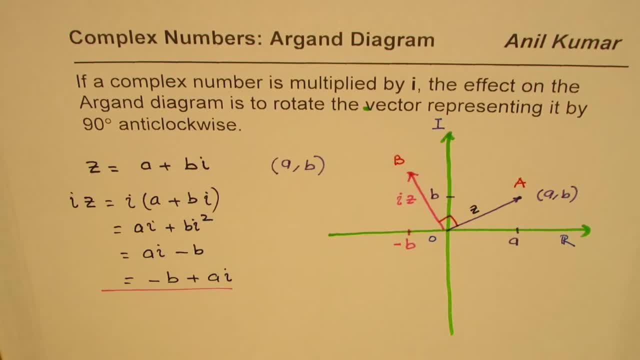 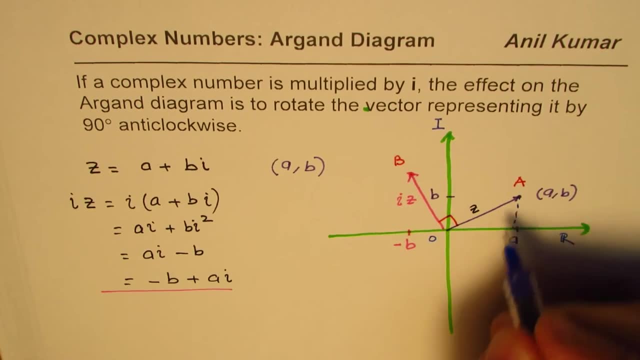 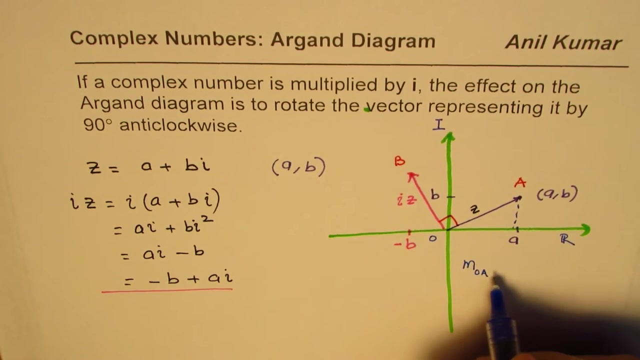 The slope of this line is how much? Let's calculate that slope right. That should help us to find the angle. So the slope of this line is, let's say, slope M of the first vector, where, say, OA is equal to the height. 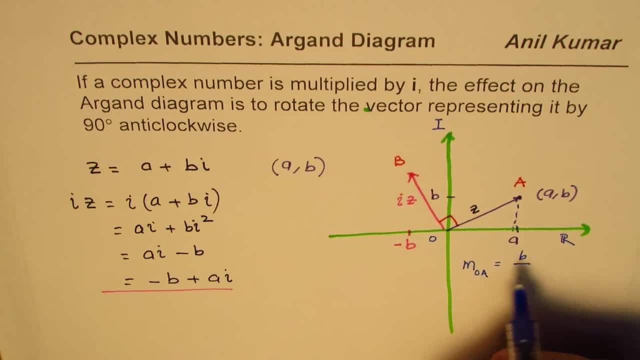 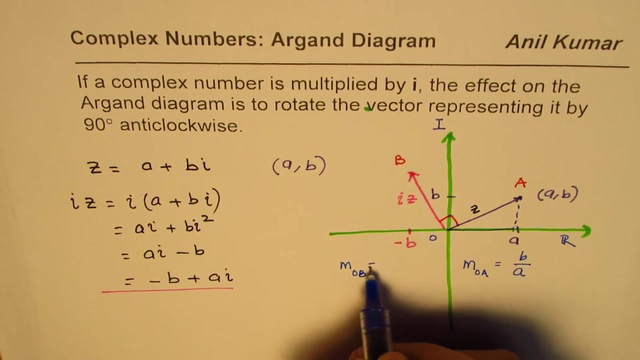 This is the opposite side, which is equal to B over the base, which is the R real coordinate A. So the slope is B over A. On the other hand, what is the slope of OB? Now, in this case, if you find the slope of OB, 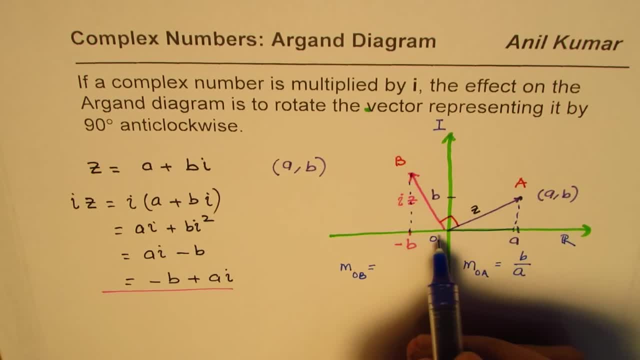 then it is the height. In this case, the height is equal to A, So this is equal to A, A, A, A. And the base length is minus B, So the slope of this OB is minus AB. Now what happens when you multiply the two?